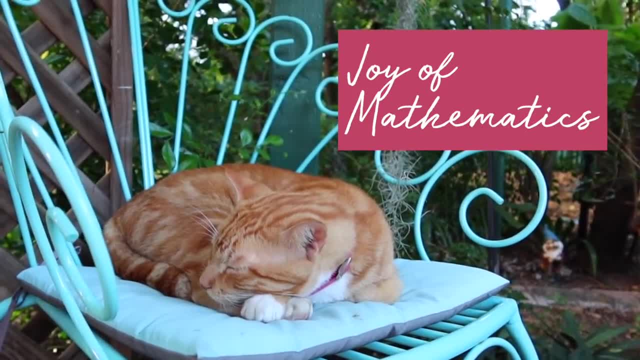 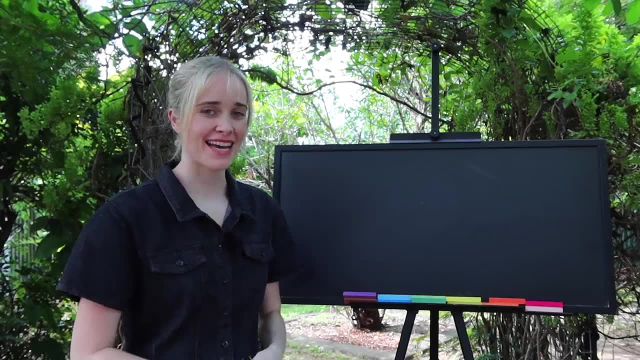 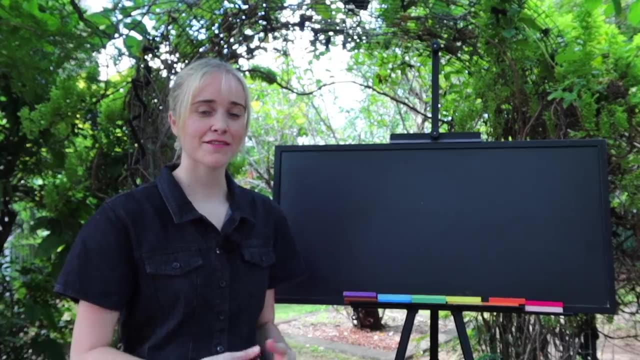 Hi, I'm Toby and welcome back to The Joy of Mathematics. It's been a minute since I filmed one of these, but I'm so glad that you're joining me again today for a relaxing journey through mathematics. I'm going to run some things across the bottom of the screen that we will come to. 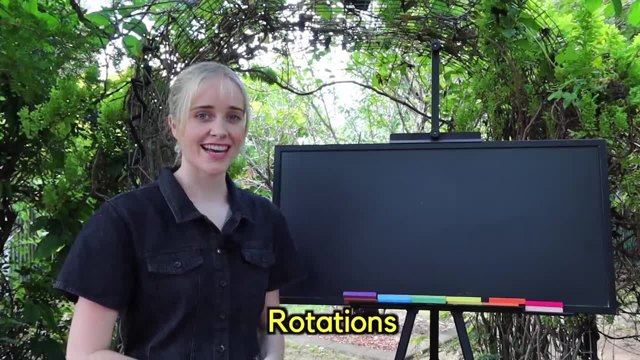 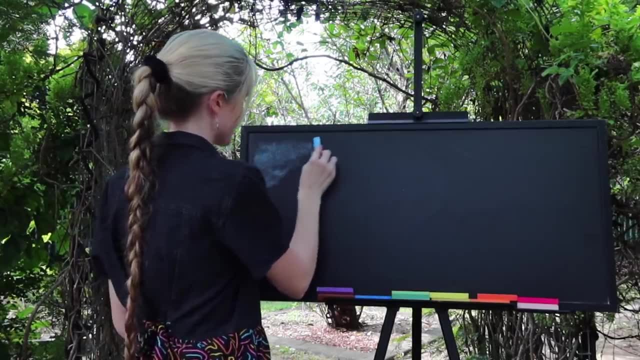 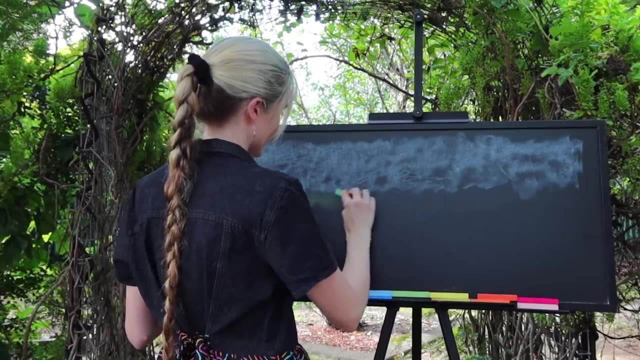 understand in this video, but mostly we will be learning how to escape from reality. Some people do this through drawing, painting, reading or playing video games, but we are going to get a private tour of an imaginary world with the help of my imaginary friends Before I. 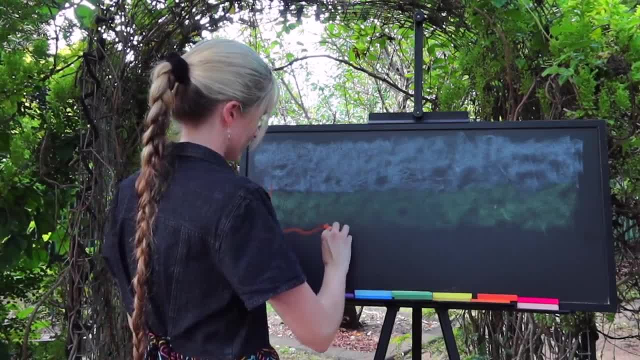 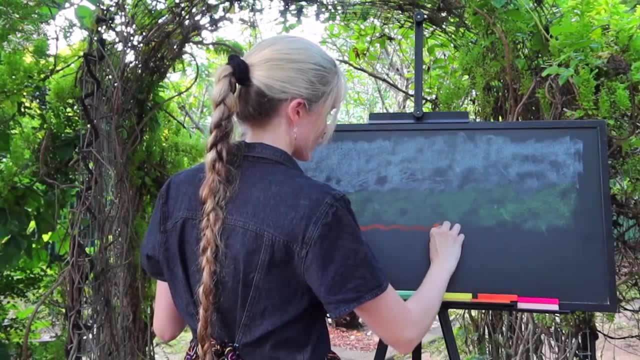 introduce you. let me tell you a story. When I was six years old, I remember a kid in my class at school saying that there were secret numbers that only he knew about. He said that the teacher had a secret number that only he knew about. He said that the teacher had a secret number that 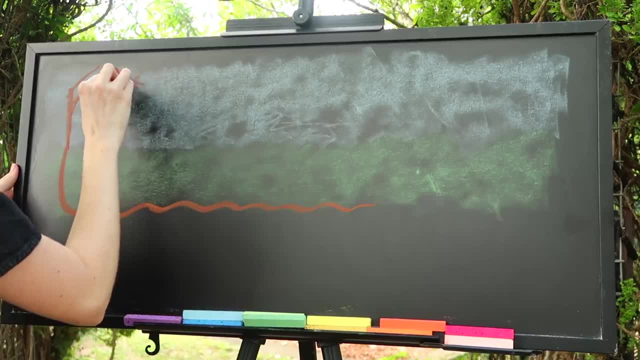 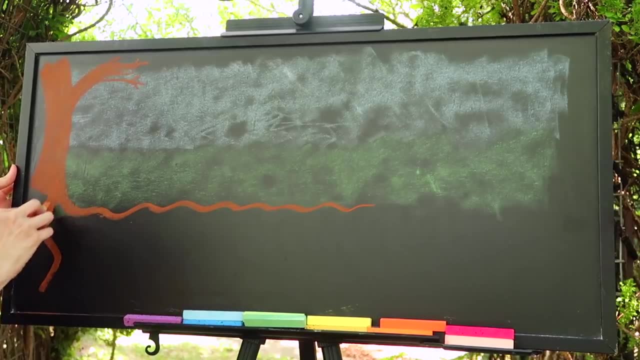 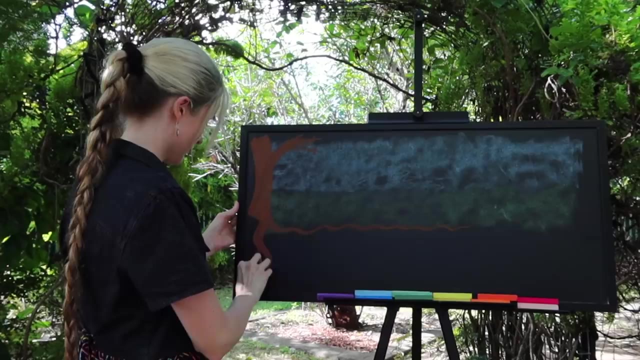 told him about them after class, that they were less than zero and called negative numbers. I was doubtful. I hadn't ever heard of such things. I thought that if it was true, then the teacher surely would have told all of us. Maybe I felt a little hurt that she had picked a favourite. 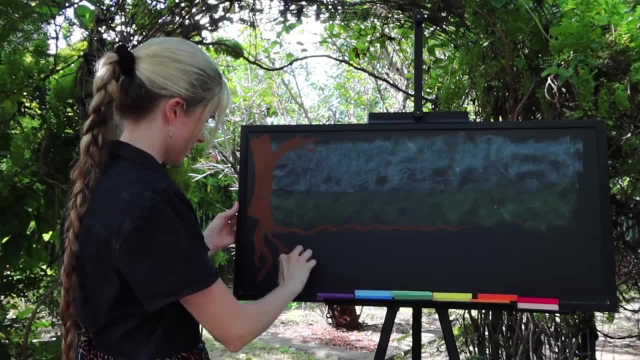 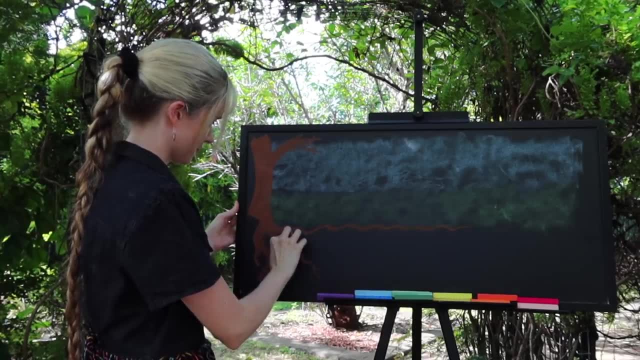 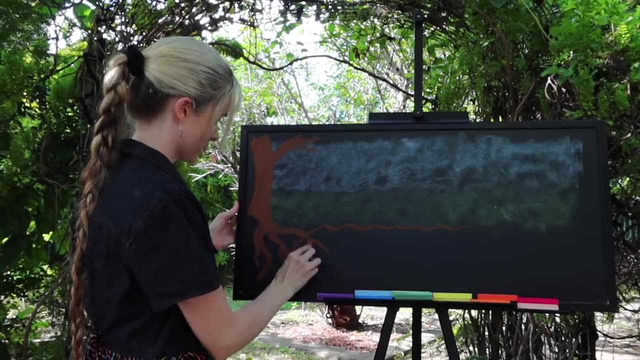 student or that I was missing out on something. Perhaps that's why I still remember all these years later. Of course, I eventually found out that negative numbers were real, but I had another similar experience several years later In high school math class. we had a relief teacher one day. 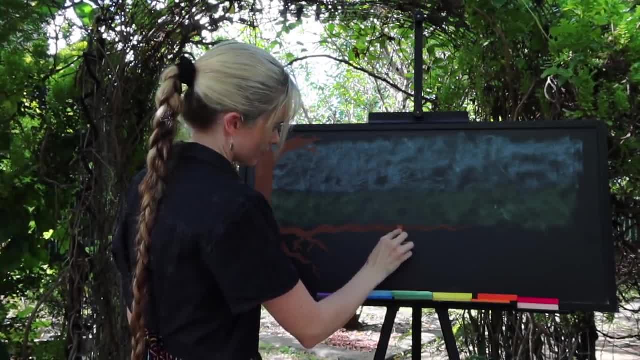 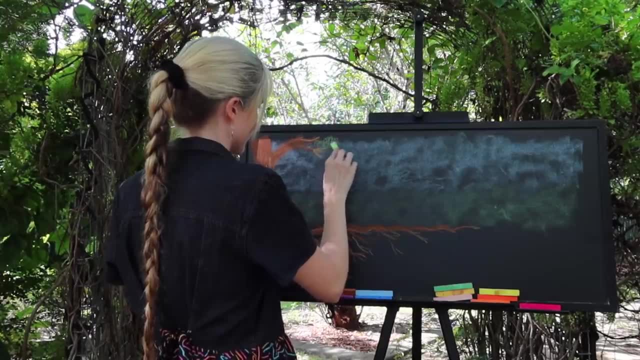 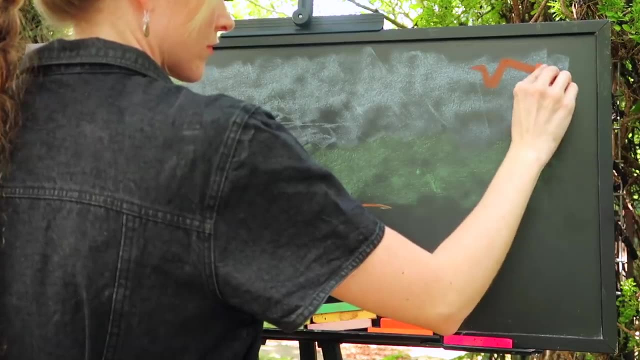 I think it was the careers counsellor. He spent the start of the hour following our teacher's lesson plan but towards the end veered far enough, off course, that he said: Have you guys heard of imaginary numbers? We hadn't. After the first animated strokes, he drew large axes and labelled one real and the 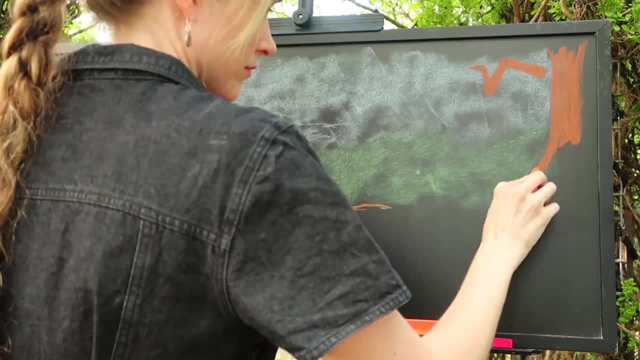 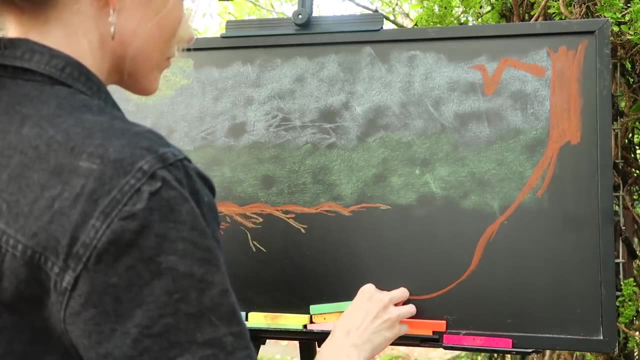 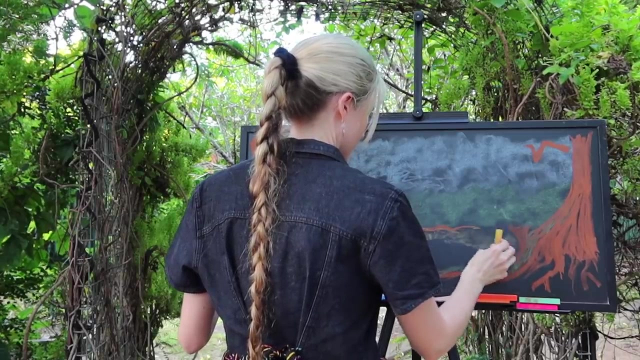 other imaginary. After that class I felt pretty mind blown. Maybe I was yet to really understand them, but that was the first I heard of these mysterious new numbers. I had again experienced my view of numbers being expanded. A long time later I would realise. 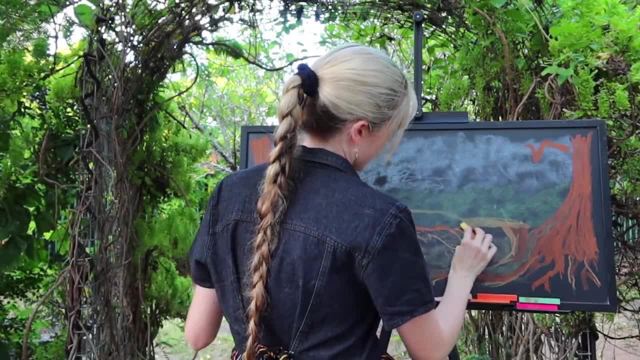 that negative numbers and imaginary numbers were just ideas of my own, and I soon realised that, as much as a dream, I'm actually in a dream. It's easy to ask yourself what kind numbers are in fact similar in the way that they extend mathematics They are. 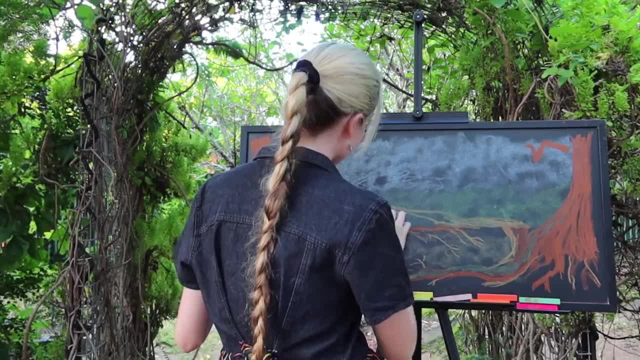 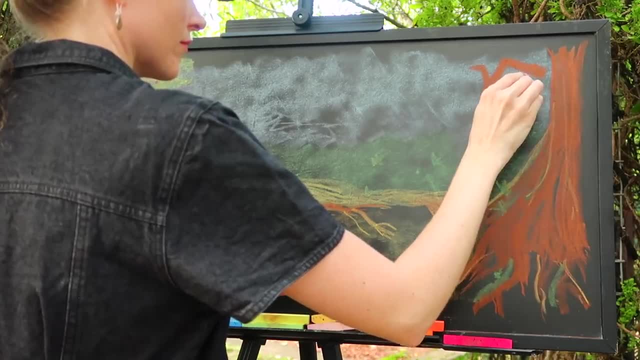 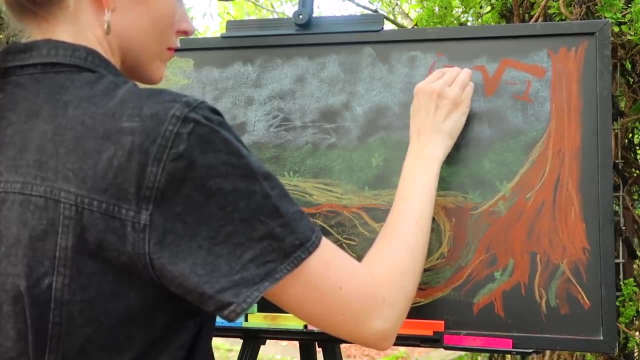 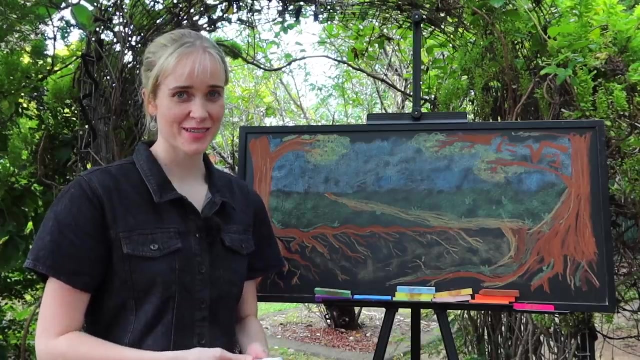 both somewhat intangible ideas that prove to be useful. Where the negatives come from asking what 1 minus 2 might equal, the imaginary unit, i comes from asking what the square root of minus 1 might be if it existed. Now, it's in the best interests of you and I to acknowledge that we live in the 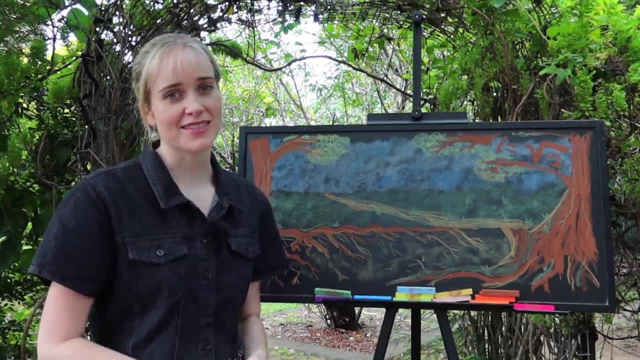 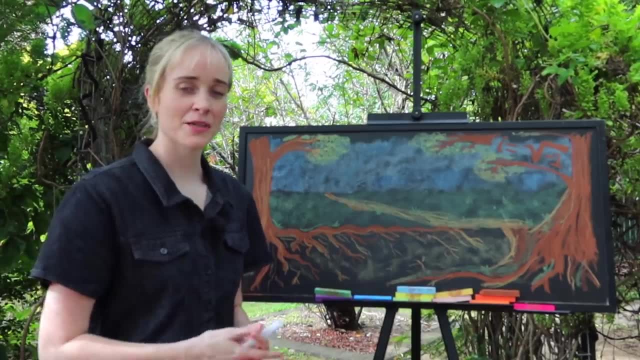 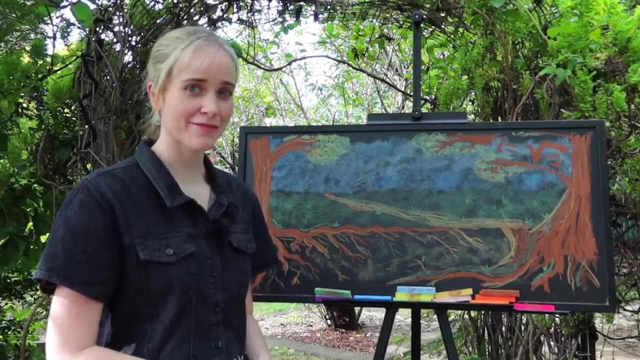 real world and our actions have real consequences, so we should try to be nice to each other. I will introduce you to my imaginary friends now, and, whilst this isn't a popularity contest, we will want to keep track of how many imaginary friends we have. At the moment, we haven't met any, so we can write I. 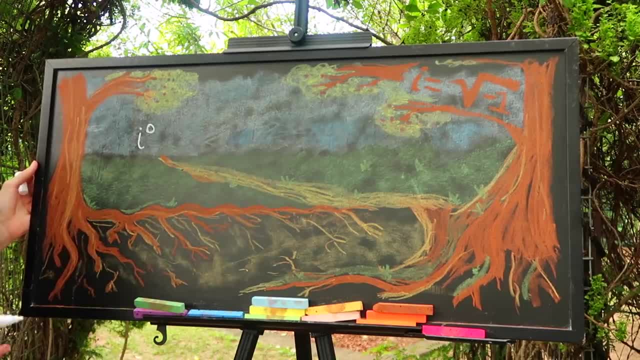 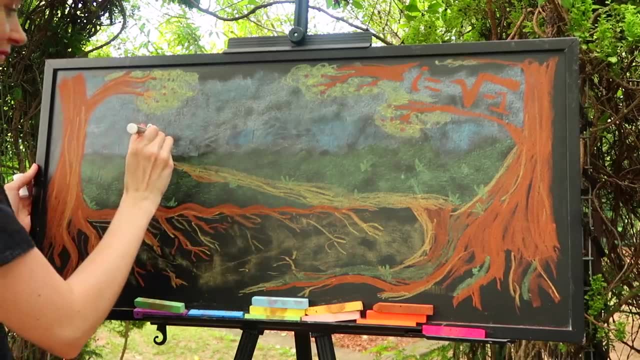 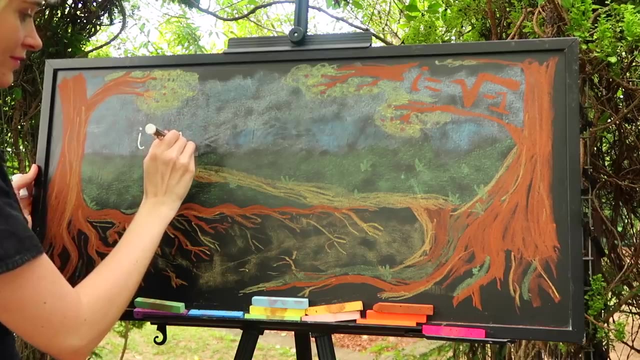 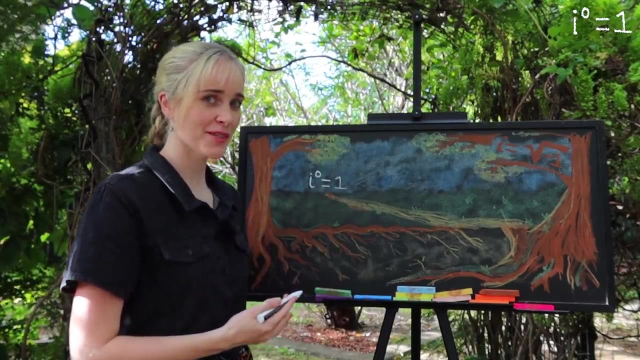 to the 0, and it's one of those quirky little mathematical facts that anything to the power of 0 is equal to 1.. This solution is our passport and since 1 is a real number, we're not going anywhere and we have to stay out here in the real world. 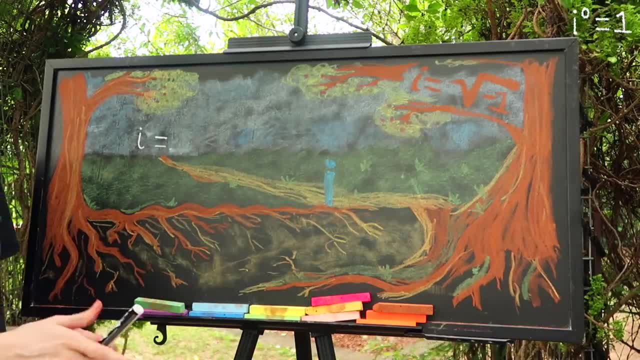 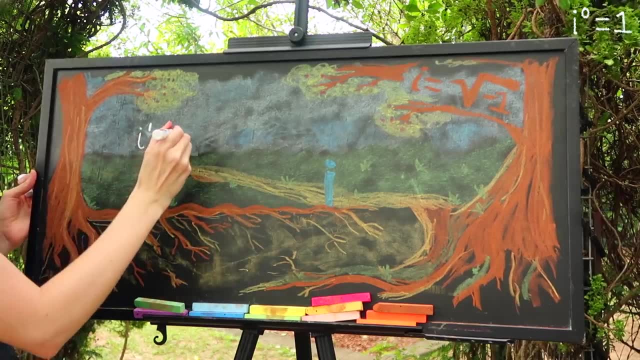 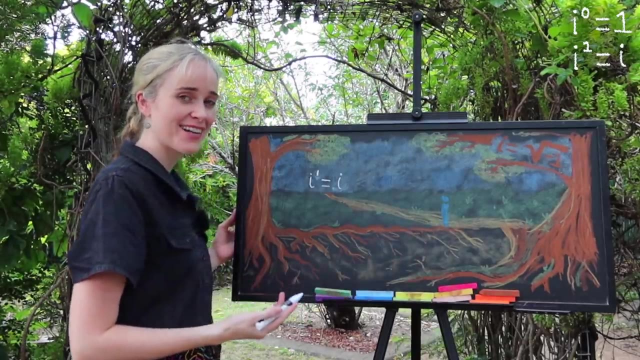 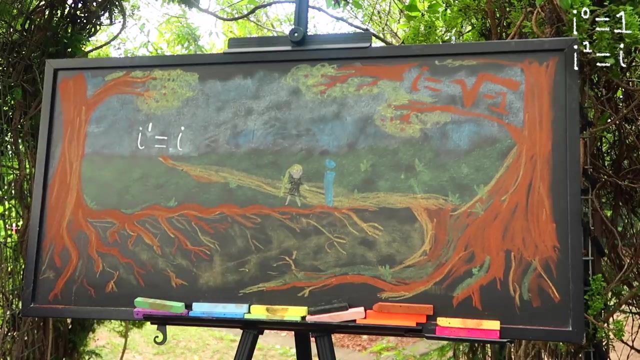 you, But meet my first imaginary friend, Ignatio. With him we have I to the 1, which is equal to I. So with our first friend we can now travel from the real world to the imaginary world. It's wonderful in here, but now I'm trapped. 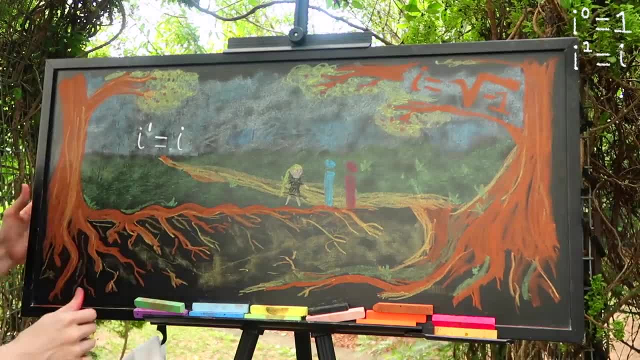 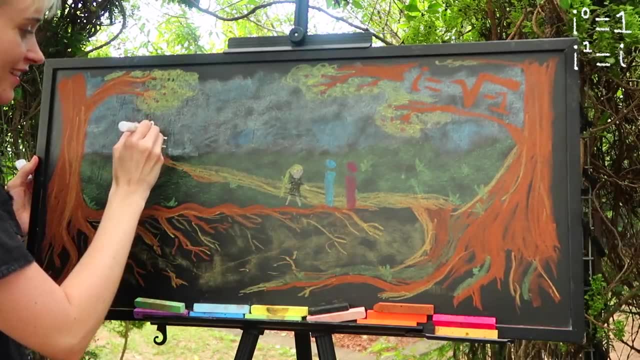 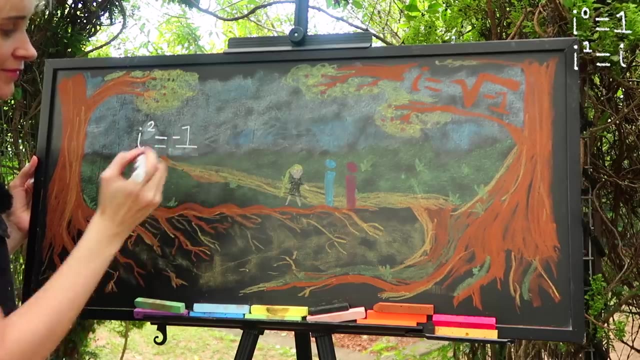 How can I go back to reality? My second imaginary friend, Ignatio, is also a really cool. He made his first friend. Iguana can help With two imaginary friends. we have negative one. I'm back in the real world, but this is the negative real world and it's so sad. 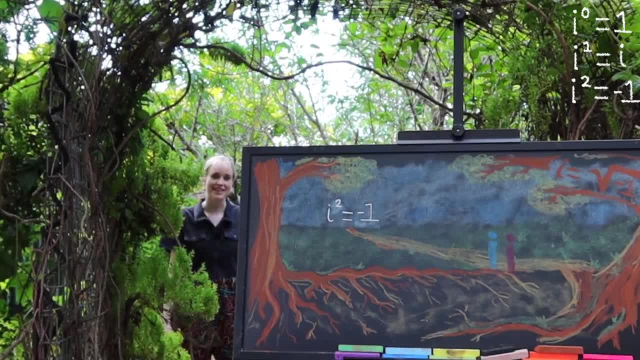 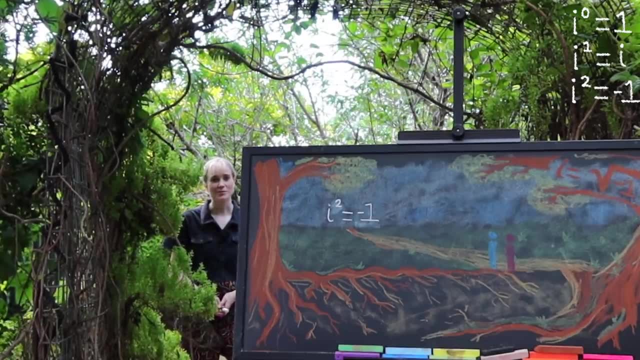 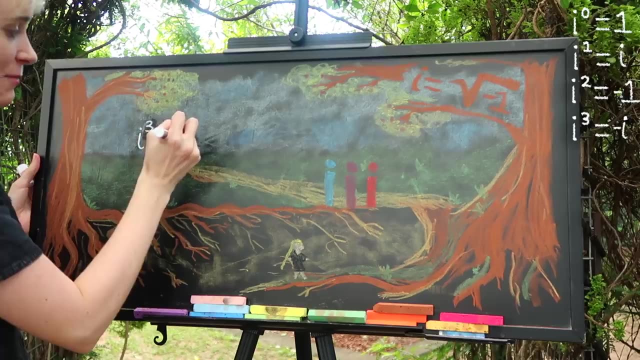 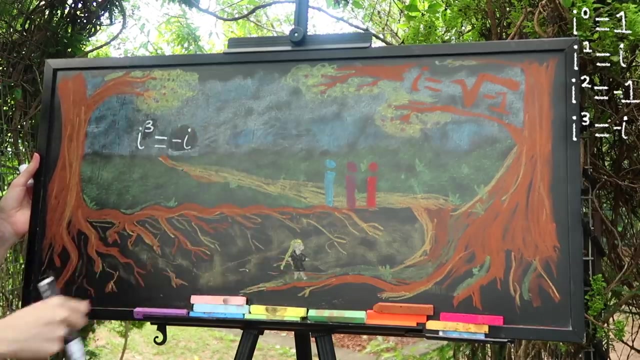 out here. I could get help from a real friend who is negative, such as minus one, but there's not really anyone out here. I could instead get help from two more imaginary friends. With three imaginary friends in total, we are taken back to the imaginary world, but we end up being underground. And a fourth imaginary 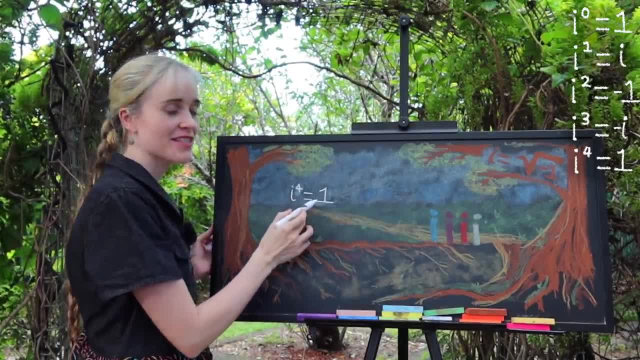 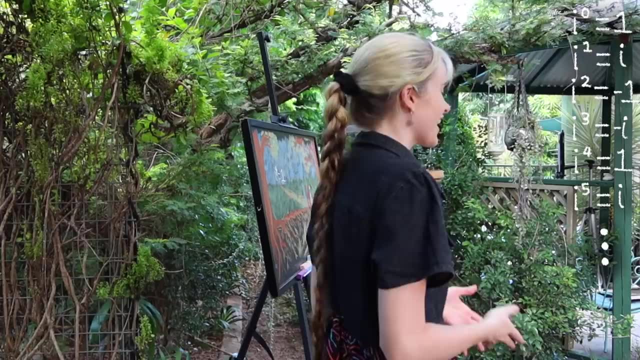 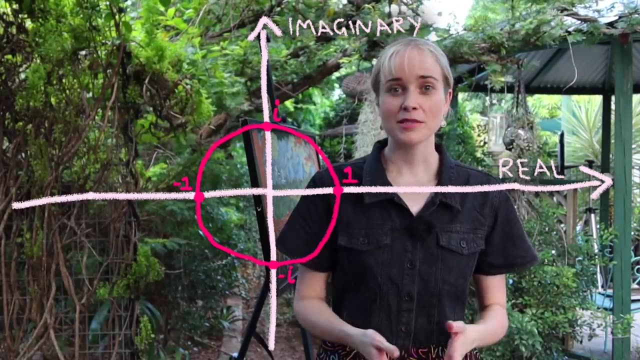 friend in total will bring us back out to the positive real world right where we started. This is all you need to know to travel between our world and the imaginary world. We can show our story on a map where we're jumping between the points 1, i, minus 1 and minus i, And that 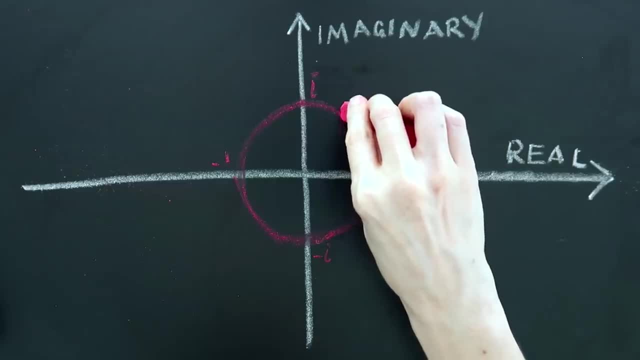 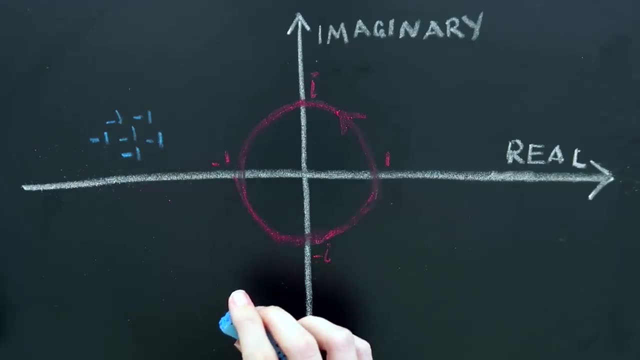 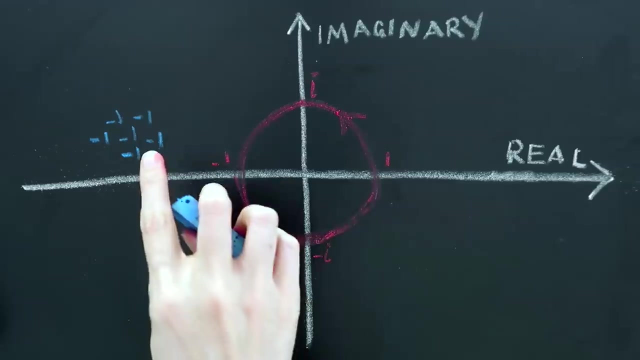 is because multiplying by i is a rotation of 90 degrees. If the friends we met had been a gang of negative numbers, then we would have toggled between 1 and minus 1.. This flipping shows that multiplying by minus 1 is a rotation of 180 degrees. 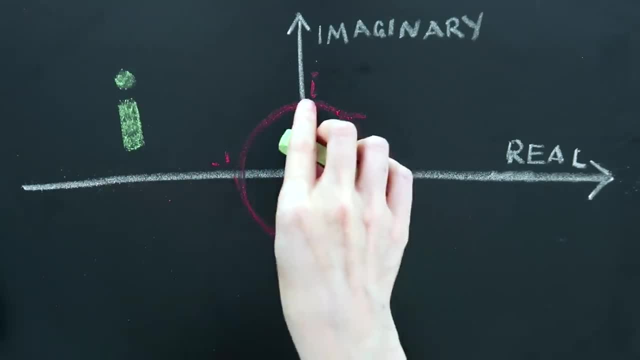 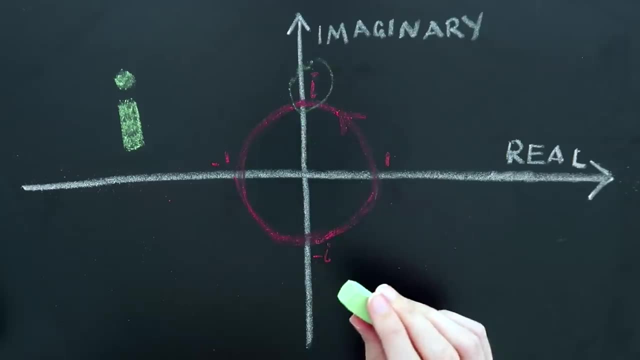 But an imaginary friend takes us to a pit stop in between to have a timeout from reality. Because multiplying by i is a rotation of 90 degrees. then if we do it twice we get to negative one, and if we do it four times we get back where we. 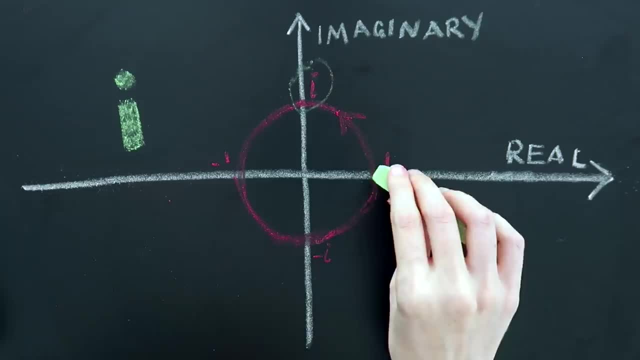 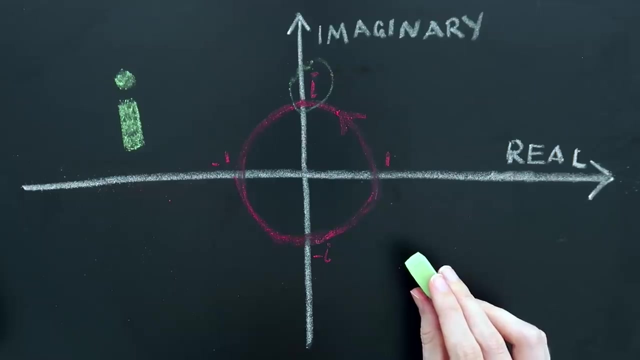 started. We could, of course, go the other way as well. We would see a clockwise rotation of 90 degrees if we multiplied by minus i. This ability to multiply and move around in a circle is what makes imaginary numbers so good at modelling things that are circular in nature or that 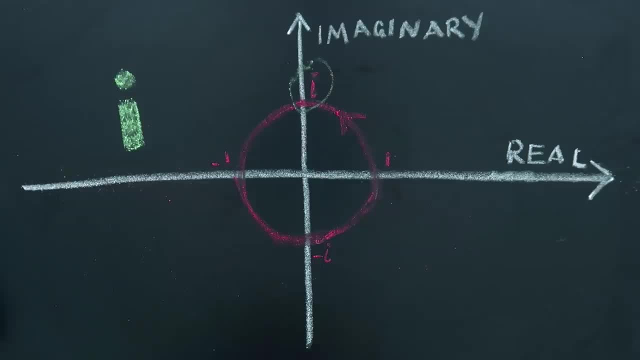 rotate And despite the name, they are not imaginary at all. Some people just have trouble seeing them And whether you want to believe in imaginary numbers or not, you can't And you can't do anything about it. You can't do anything about it. You can't do anything. 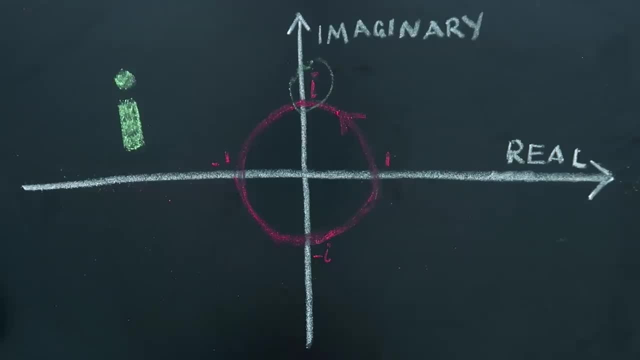 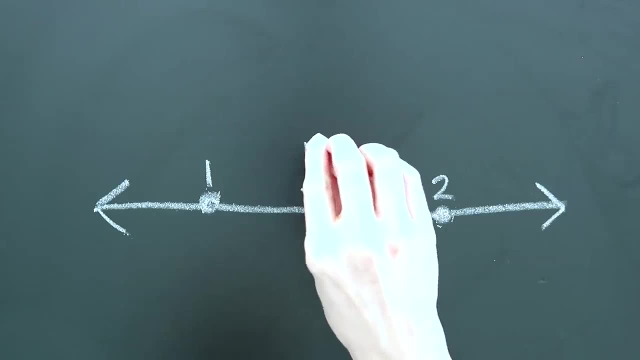 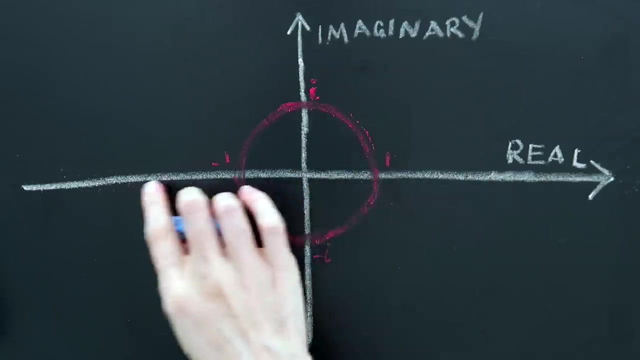 It's as mind blowing as decimals or irrationals would have been to early mathematicians. Some never got to know there were numbers in between 1 and 2. Larger friends such as 2i, 3i and 4i allow us to go anywhere on these axes, But what? 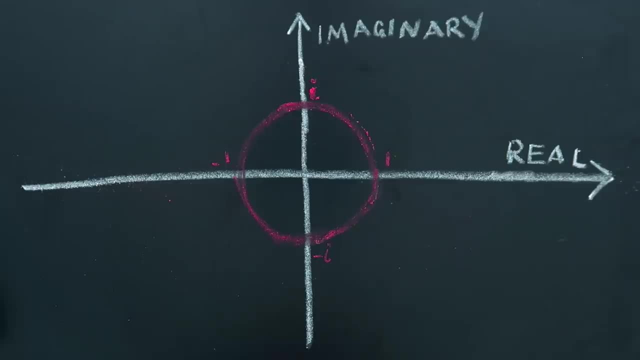 about the rest of the plane? Well, yes, we can travel anywhere we like. It's just a little bit more complicated. This is the complex plane, after all. In the rest of this region, we need two parts, a real part and an imaginary part, to explain where we are. 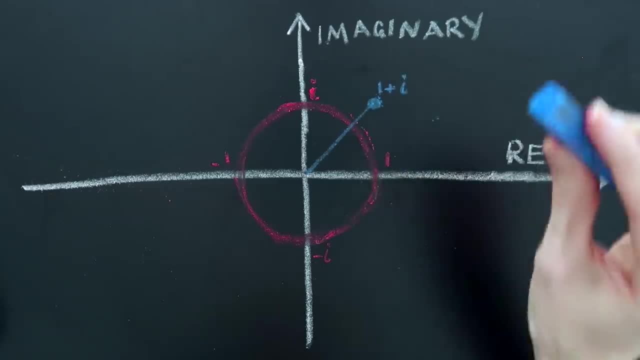 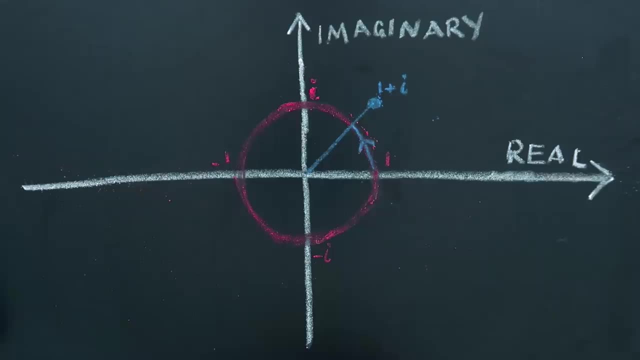 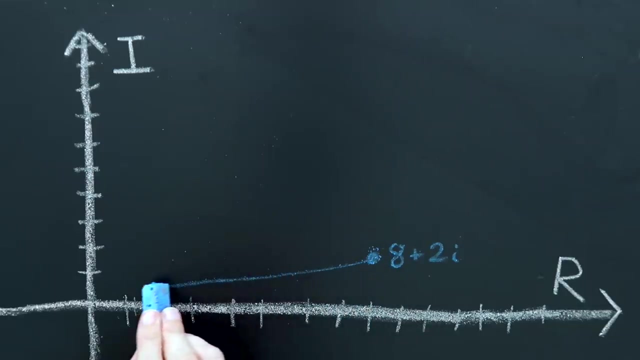 With one foot in each door here at one plus I, we are halfway between worlds, A rotation of 45 degrees. Let's see a use for multiplying complex numbers. Say, you go for a walk in the forest but you end up getting a little lost. 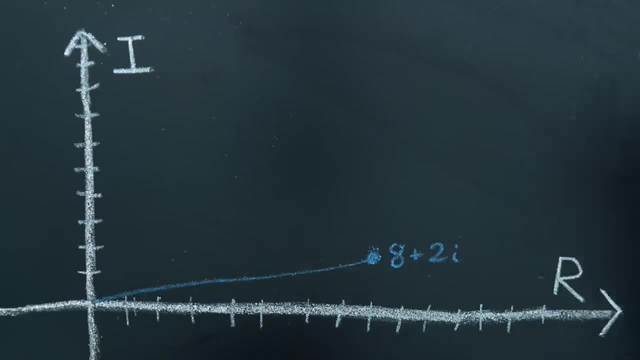 At first you walk along the path laid out in the direction of eight plus two I, But you realize this isn't right and you want to change your track by 45 degrees. How would you work this out? Well, normally you could do some trigonometry. 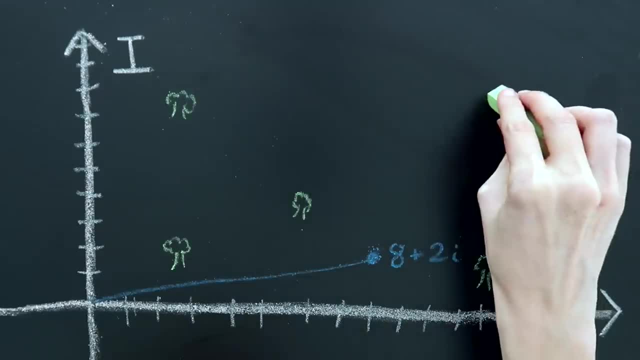 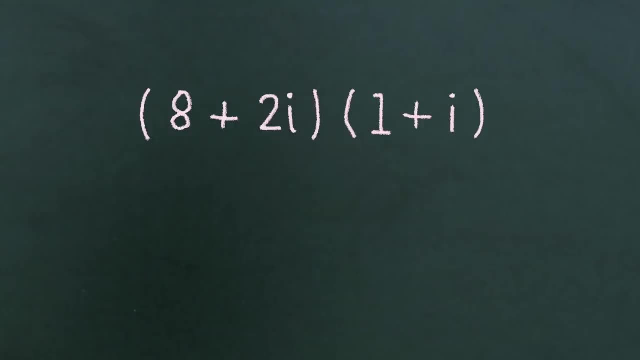 some sine and cosine. Maybe you need to carry a protractor with you to work out the angles. Or you can multiply eight plus two I by one plus I, which we already know is a rotation of 45 degrees. Eight plus two I times one plus I is equal to eight. 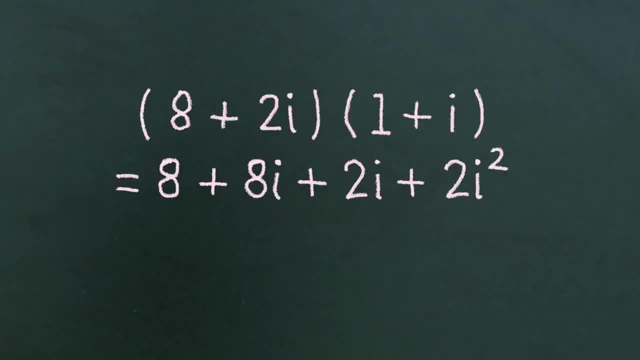 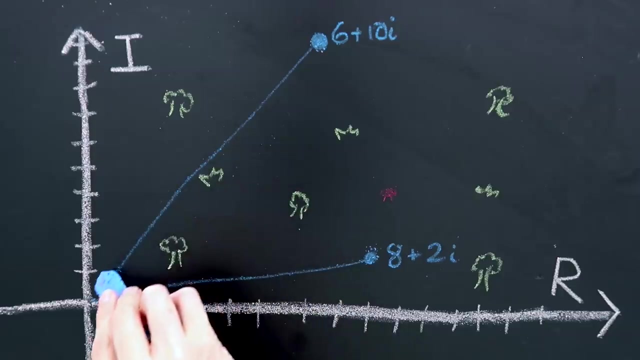 plus eight, I plus two, I plus two, I squared. Since I squared is equal to minus one, that term becomes equal to minus two and we end up with six plus two. I So walking along the path laid out in the direction of six plus two. I. 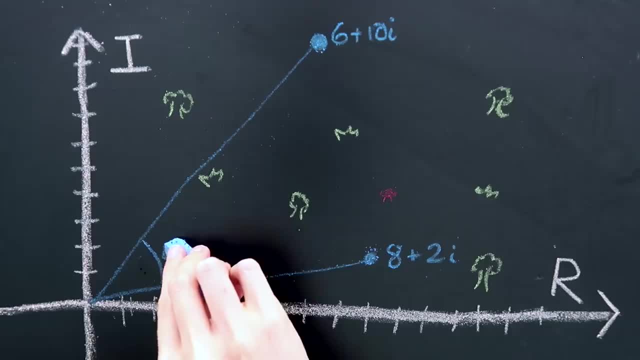 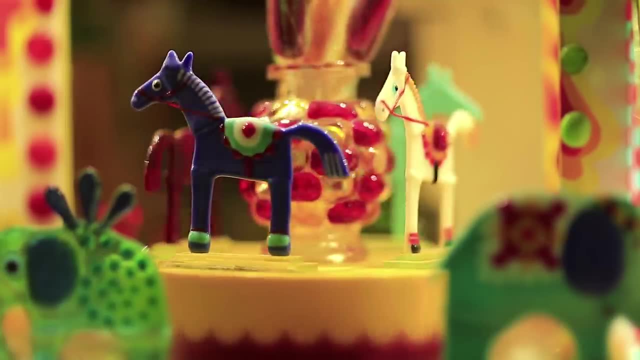 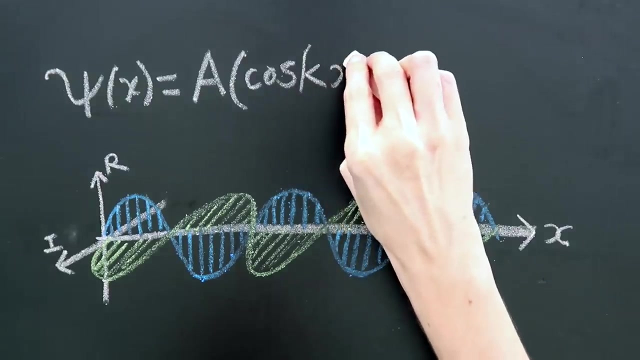 will be an offset of 45 degrees from the original path. Introducing imaginary friends has given us an extra dimension in which to travel and a useful tool for performing rotations. These friends might become a dime, a dozen as you go on in maths, but each one is still special. 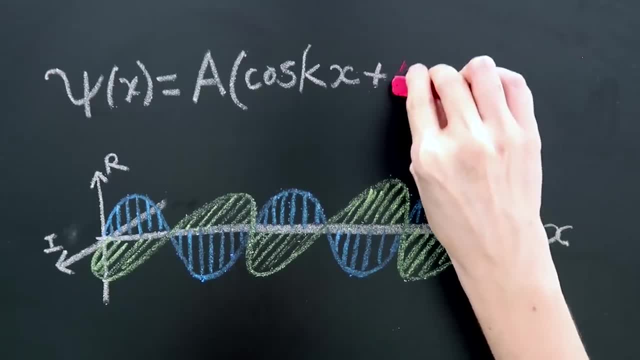 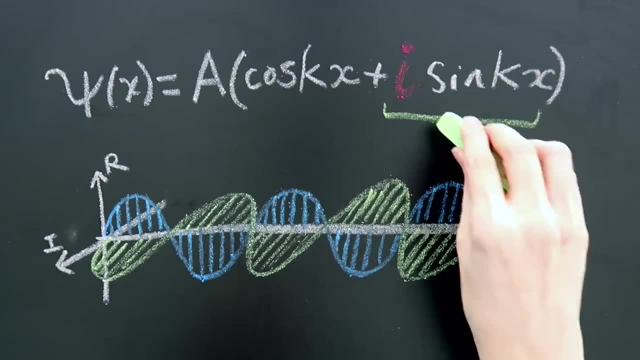 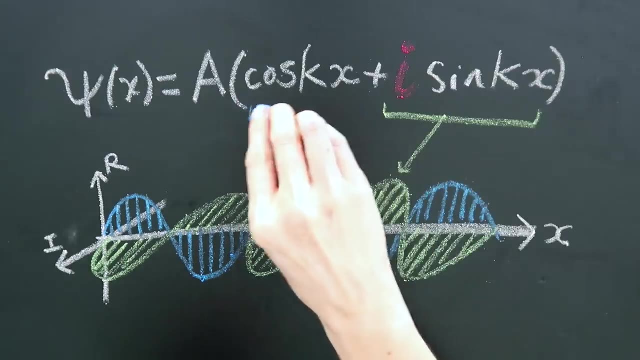 I'm proud of the friend who appears in the wave function of the electromagnetic wave. The electric field and magnetic fields are perpendicular to each other and their magnitude and time variation are correlated By assigning the magnetic wave to the imaginary part and the electric wave to the real part.